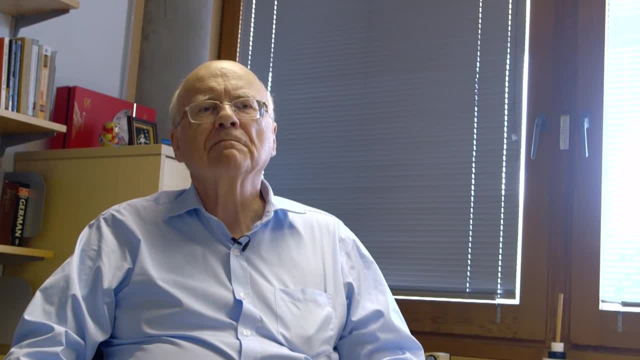 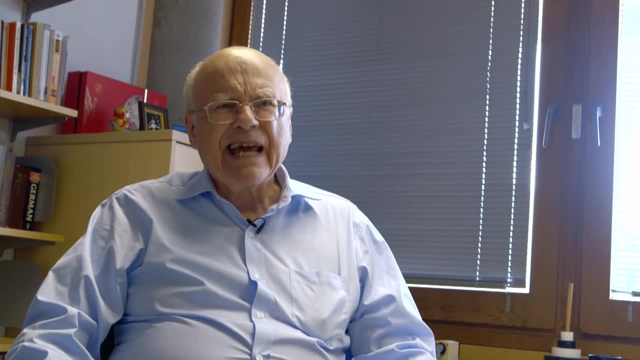 There's one thing that we keep coming back to, and it's the idea of Turing Complete. What does it mean and why do we need to worry about it? Yeah, what does it mean to say it's a language. It's usually, in this context, a programming. 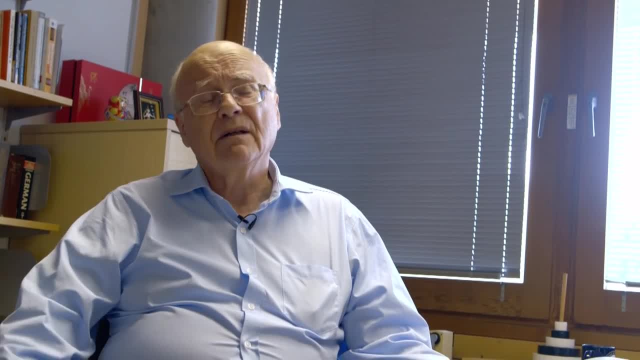 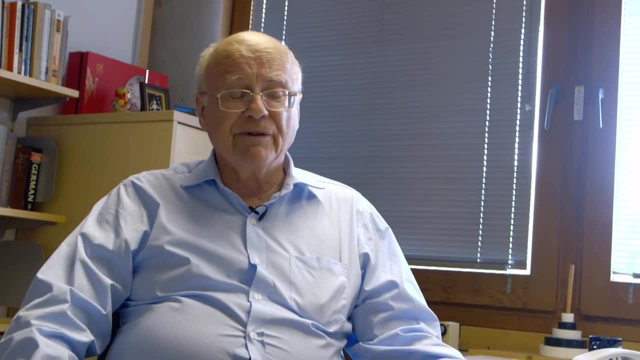 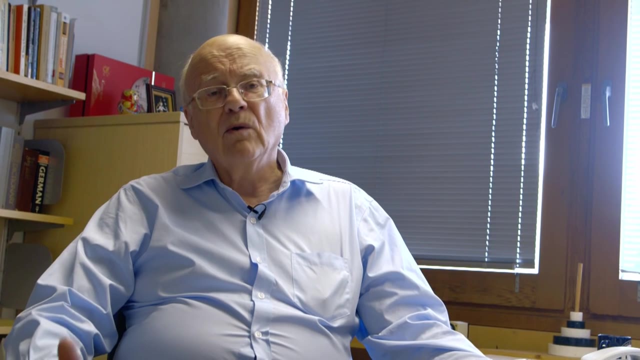 language is or is not Turing Complete. Well, obvious first example is that every programming language you're familiar with- I mean we'll refer to the usual suspects- Fortran, BASIC, Pascal, COBOL C, C++, Java, They are all Turing Complete. 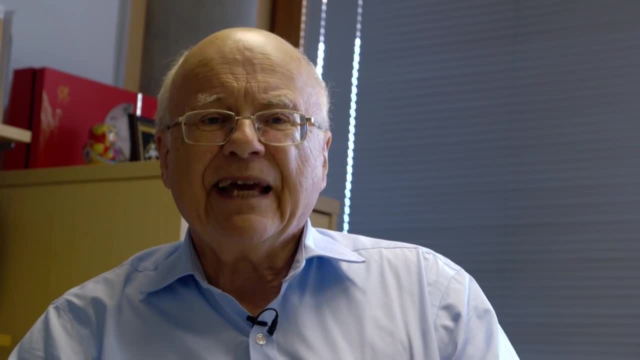 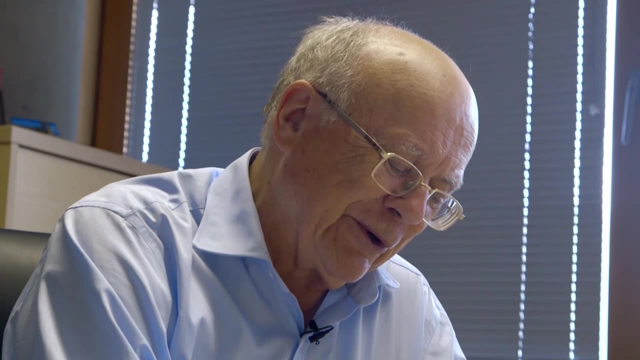 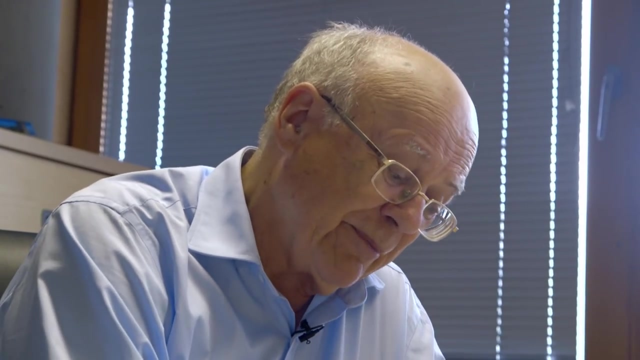 So what, fundamentally, does a thing have to be in order to be Turing Complete? And the answer is it needs to be able to do everything that a Turing machine can do. Mercifully, we have made several videos on this topic, Some from me, some from my colleague. 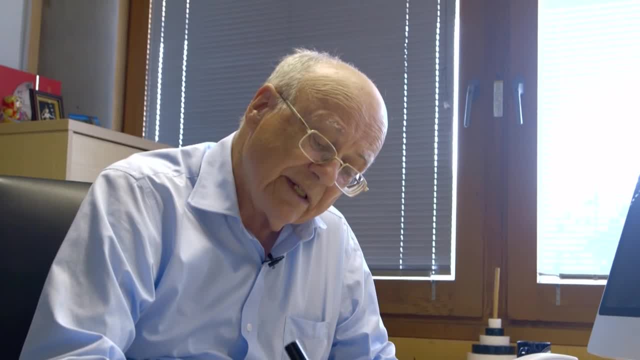 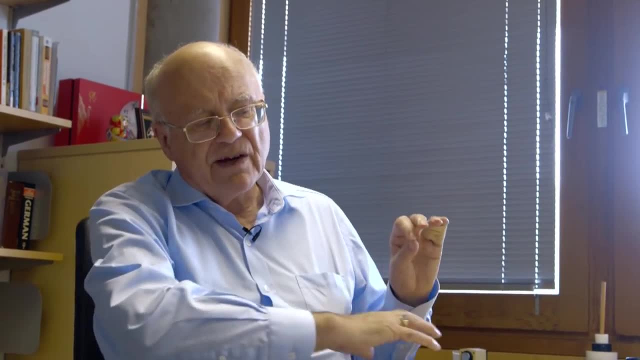 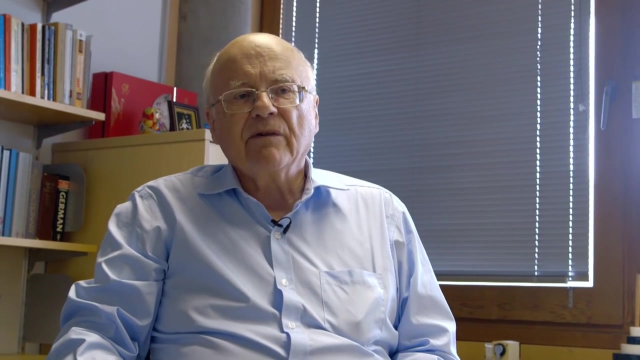 Mark Jago And we have visited quite a lot of these issues. Just to recap, a Turing machine is thought of as an endless, infinite piece of tape And it has a read-write head that goes over the top of the marks on that tape, which can be anything you like, But conventionally, to keep it very simple, you. 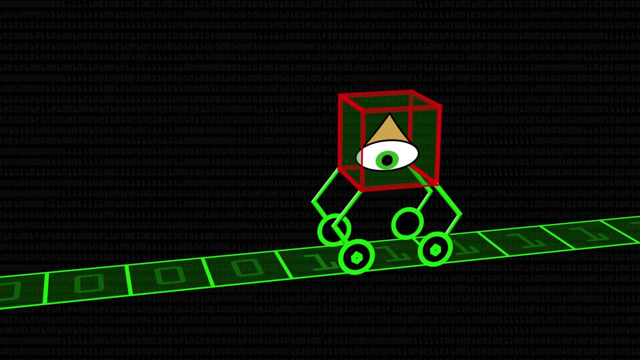 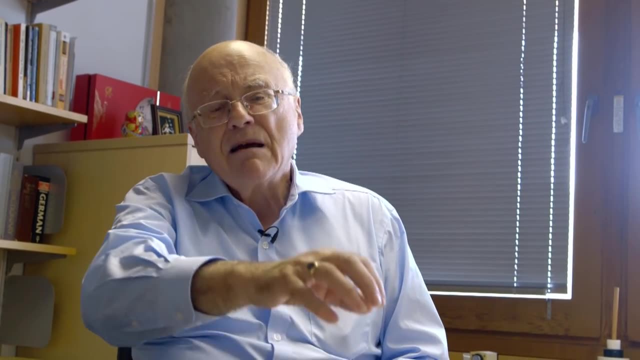 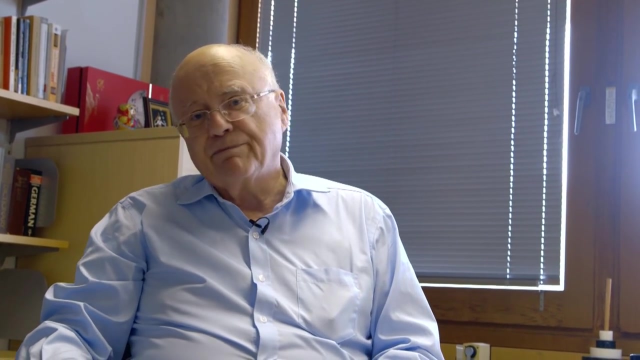 say it's zeros and ones, And you can show that just the ability to read and write on an infinite piece of tape patterns of zeros and ones is powerful enough to compute anything that can be computed. Admittedly, your low-level Turing program with all its zeros and ones may be. 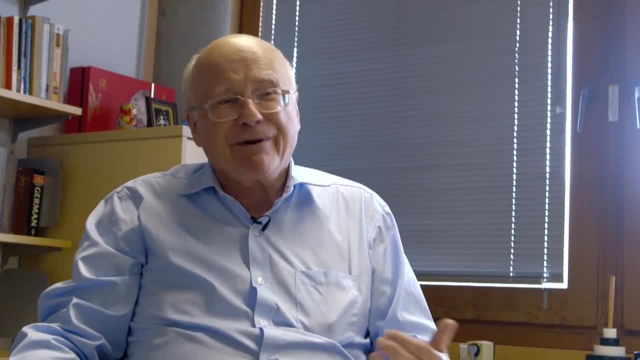 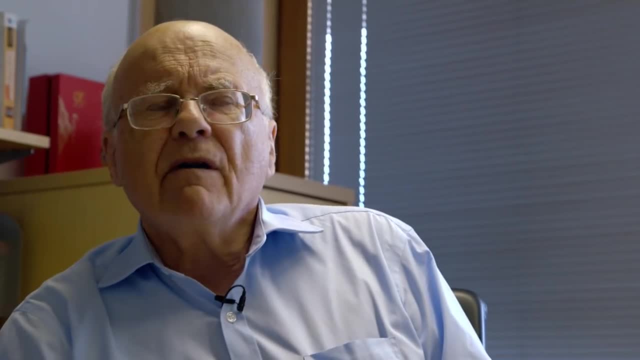 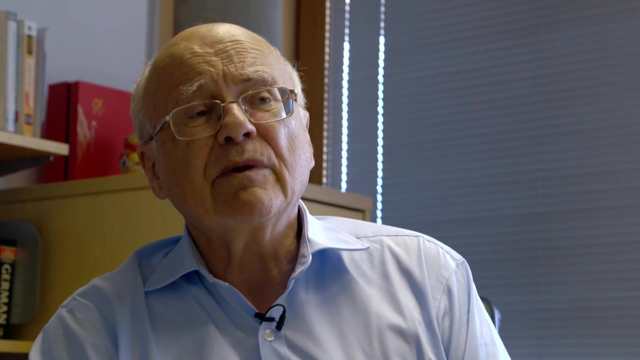 10 trillion times longer than your Comparacy program. I don't know, But in principle it can do exactly the same. Some people argue that actually, although it was Turing that made brought this all to our attention in the late 30s with the work he did, in some ways some people would say it really ought to be. 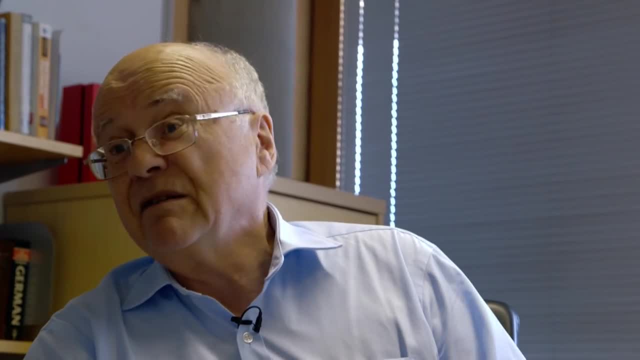 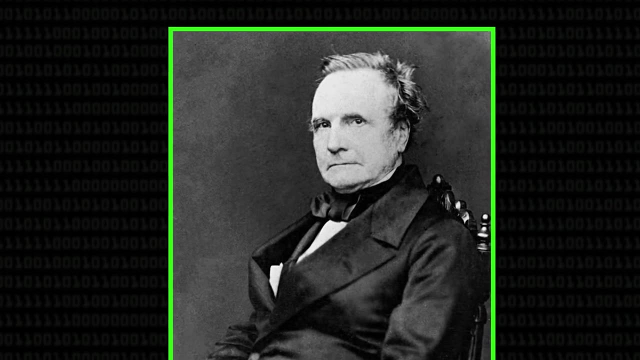 called Babbage Complete Because another UK. well, he was a computer scientist. actually, in the way his brain worked. Charles Babbage, Many of you know he started off by just doing very powerful calculating machines, difference engines. Well, going beyond that, some of you will know that 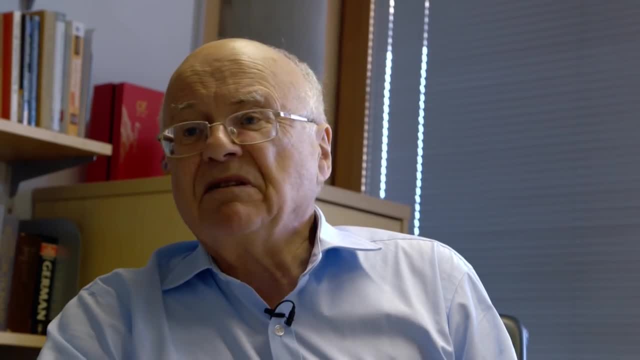 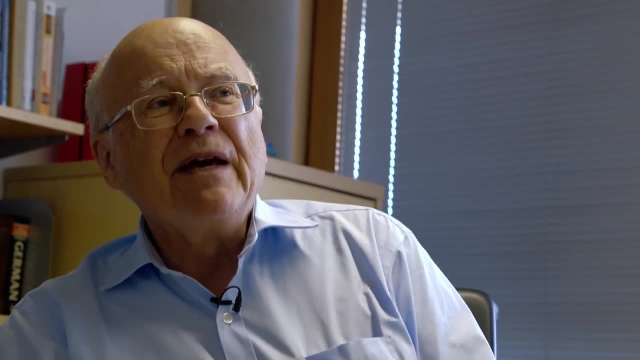 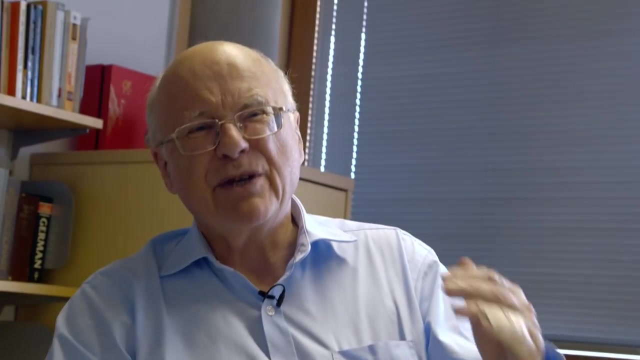 Charles Babbage said: well, that's just like a calculator that you have in your top pocket But it weighs about 10 tons and full of cogwheels. But even just using cogwheels. he went on and said: I want to do something that really can compute in the way that a human can do, And the one thing he 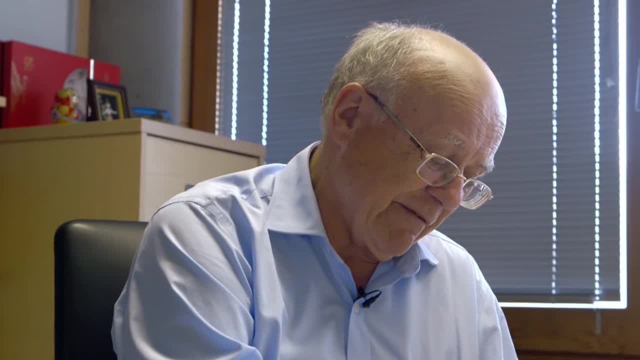 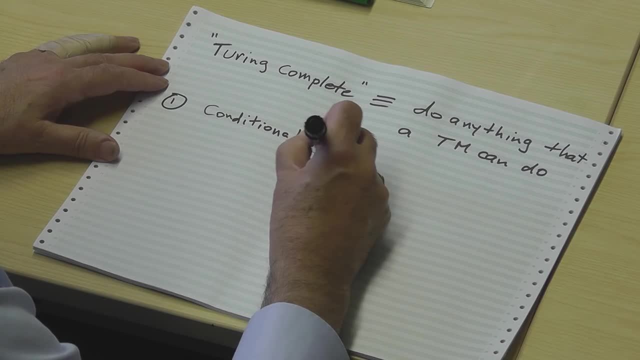 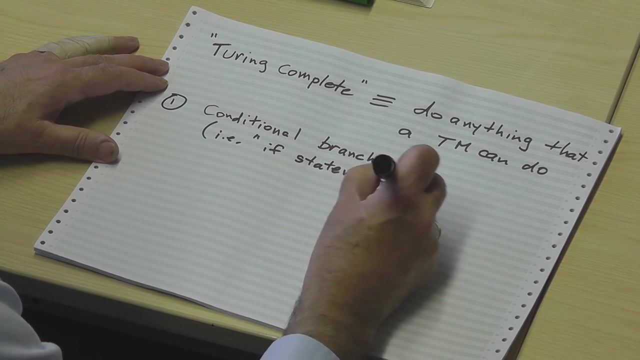 realized straight away is, to make it really powerful enough, you must at very minimum have what was called in those days conditional branching If-statements. You've got to be able to say that I'm going to look at a certain cell on. 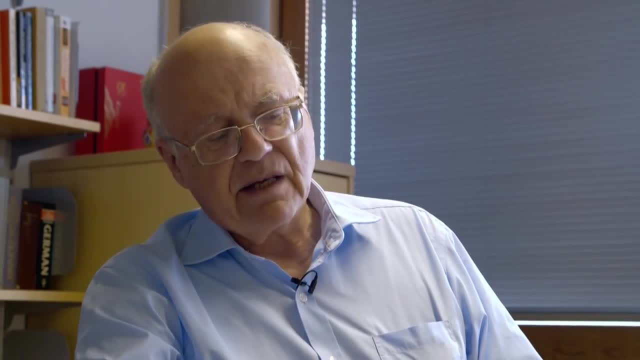 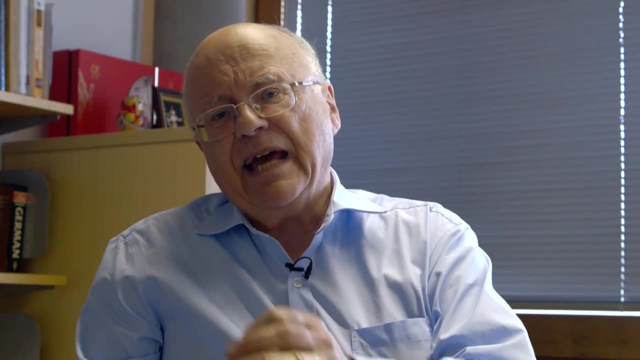 my tape, And if it's got a 1 in it, I'm going to do this thing, And if it's got a 0 in it, I'm going to do that thing. So it's this sort of two-way choice that an if-then-else. 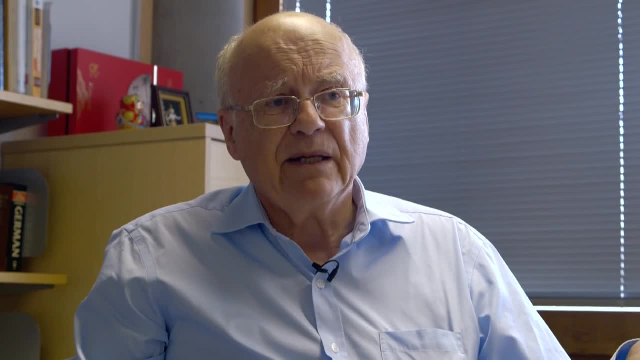 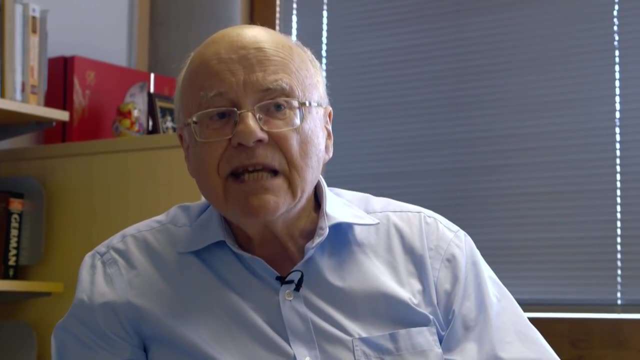 statement can give you. And he said it's absolutely vital to be able to do that Because very often the computations that humans do depend on the precise nature of the data they are given. So if you want to create something, let's just say that you need to put some. 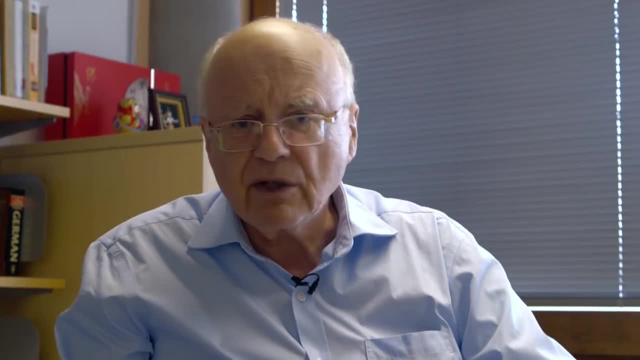 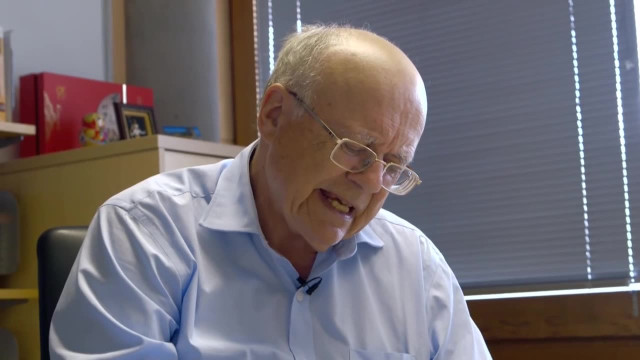 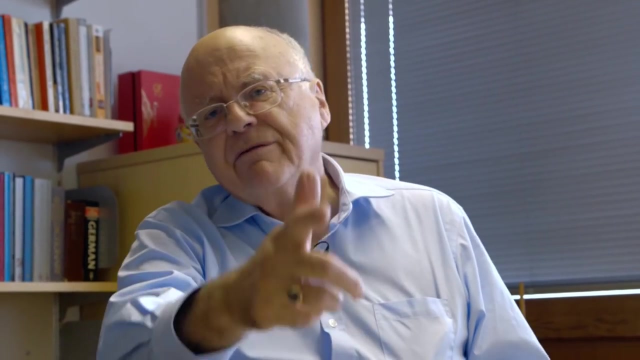 some data will send you one way, some data will send you another. So this conditional branching is absolutely vital And as a sort of kind of result or side effect of that, it also implicitly means that you've got to have the ability to go to somewhere different in your memory. For example, you might be 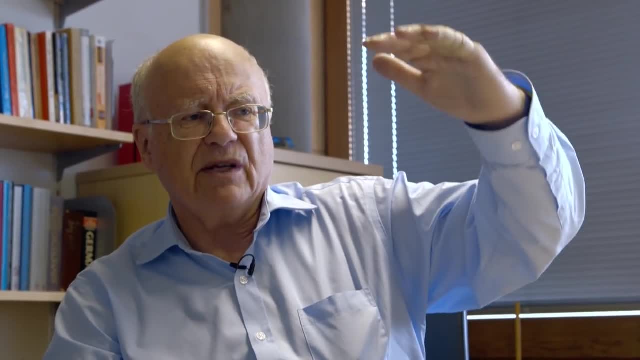 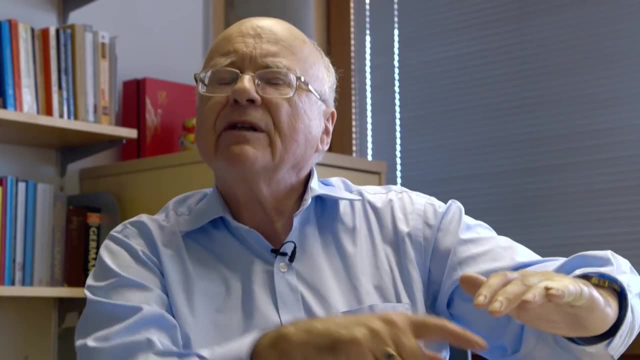 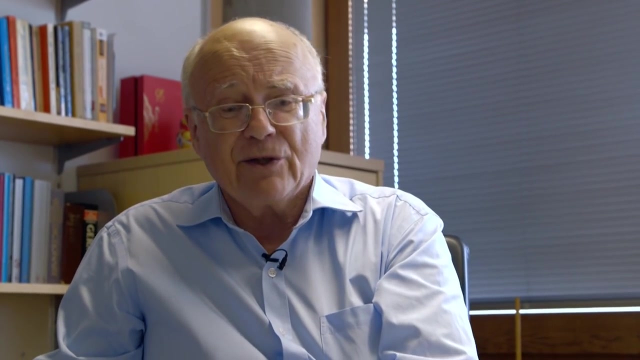 saying: if this condition is true, then I carry on with the sequence of instructions that immediately follow, But on the other hand, if the else statement is true, then I have to go off somewhere else and do something different. Now, all our undergraduates, we absolutely do not encourage the raw use of go-to's, because 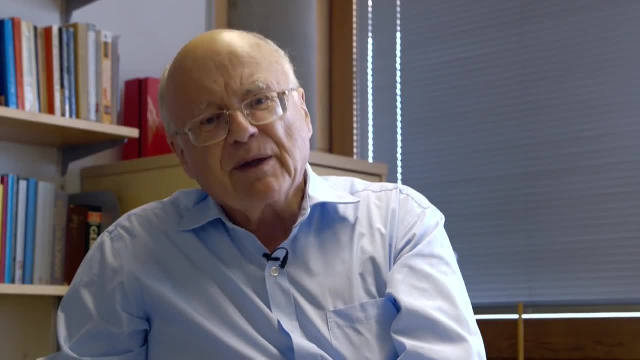 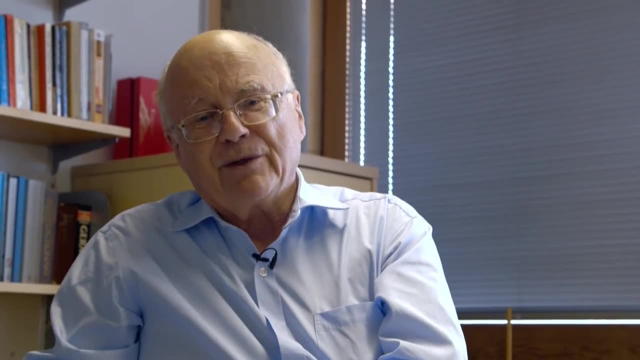 it's not good well-structured programming. But those who have done assembler will know that under the hood you can't avoid it. You really do have go-to statements which say: I'm here at location 88 or whatever. now jump off to. 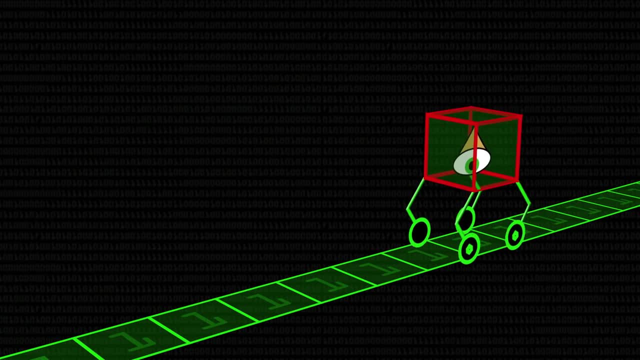 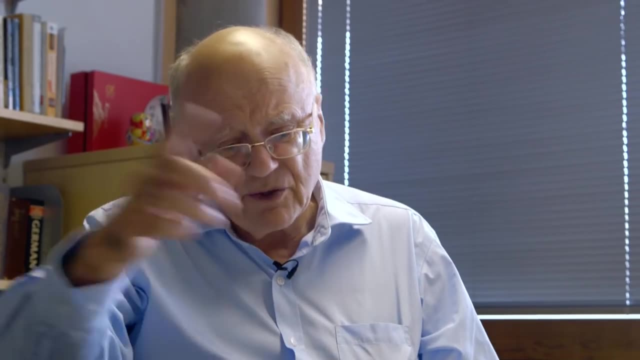 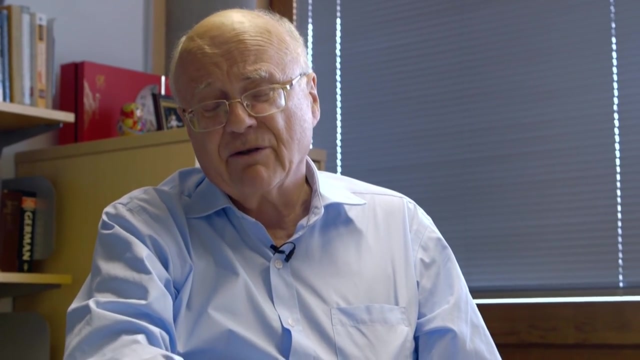 location 200.. So, if you like, the conditional branching implies a go-to in that you might stay in this part of the tape. you might jump off somewhere else. We've seen on the Turing Machine videos: it's perfectly possible to get your read-write head chattering across the.